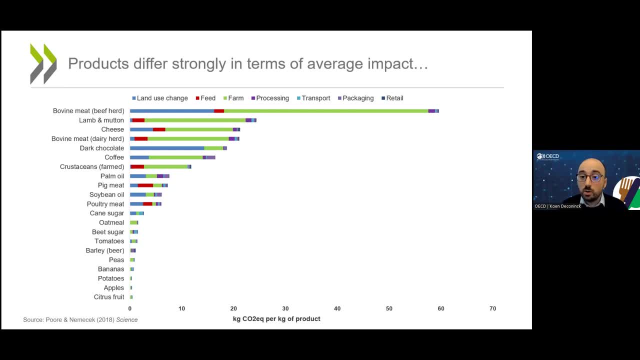 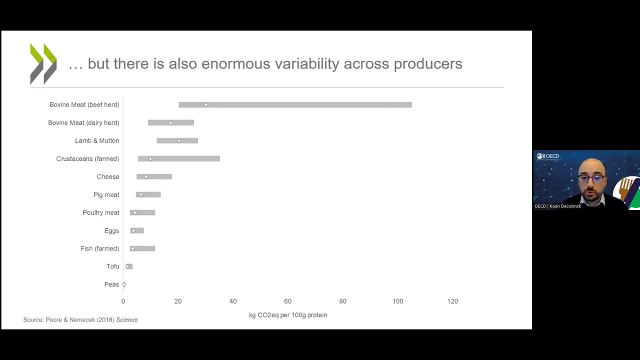 ruminant products such as beef or dairy or lamb tend to have higher carbon footprints as well. Now, this is only one side of the story, Because at the same time, the evidence also shows an enormous variability across producers. The chart here shows you two things. The white: 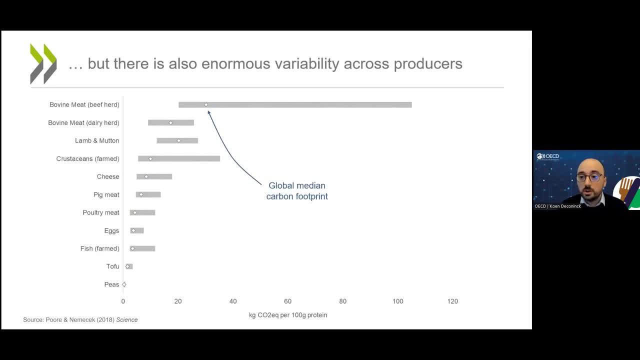 dot is the global median carbon footprint. The grey bar shows you the range between the 10% best and 10% worst producers globally And, as you can see, that range is really large, And what that means is that all of the food systems that are produced in the world are 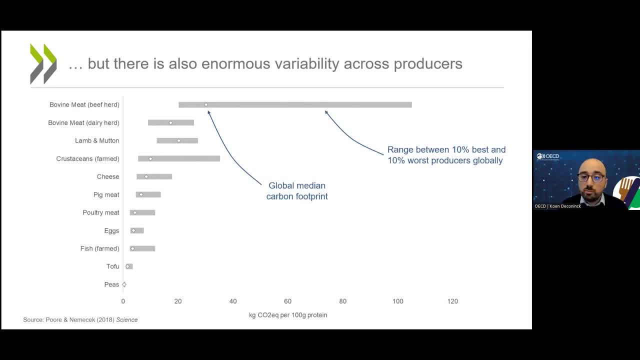 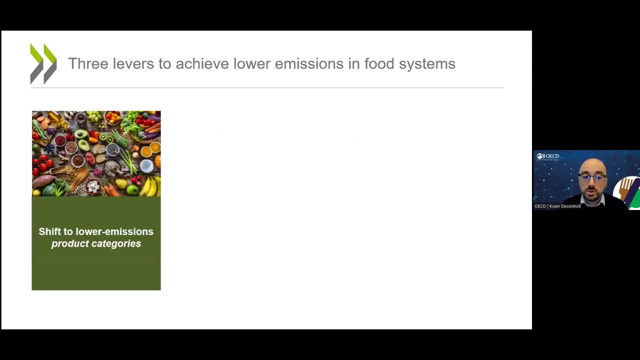 produced in the same way. If we had that information on actual carbon footprint, it would unlock several levers to achieve lower emissions in food systems. It would make it possible for us to shift to lower emissions product categories. It would make it possible within each product. 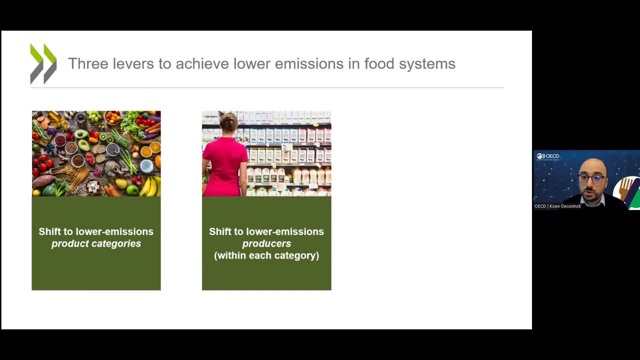 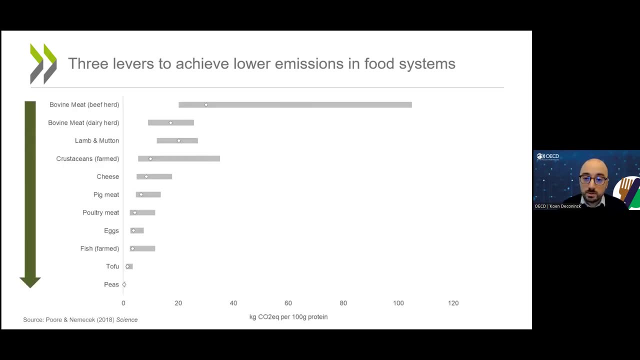 category to shift to lower emissions producers, and it would make it possible to shift to lower emissions techniques for all producers everywhere. or, in terms of the diagram I showed you earlier, it would allow us to move down this list, to move to the left within each gray bar and also to shift. 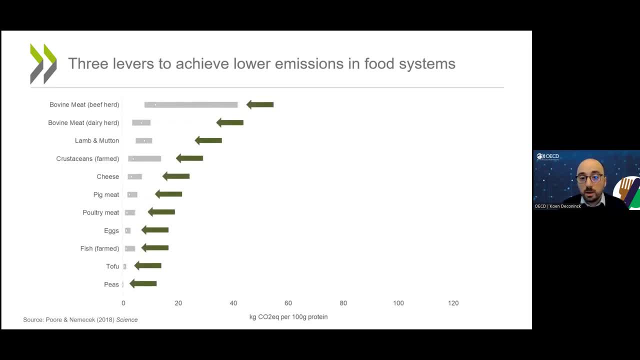 the entire distribution to the left, and there are many different approaches we could take to achieving these impacts- whether it's carbon pricing, product labeling, green public procurement, technical support to farmers and so on- and most likely we will need a mix of approaches. but the bottom line is this: whatever the approach you want to use, you can't mitigate what you don't. 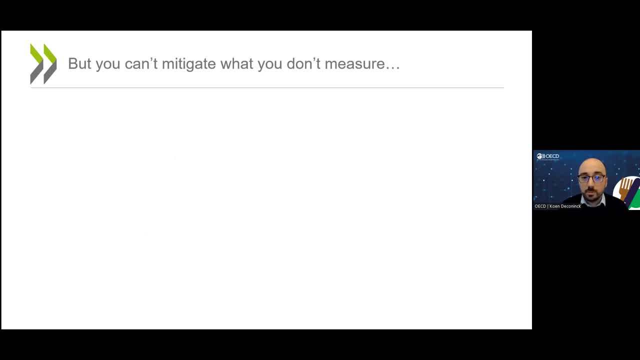 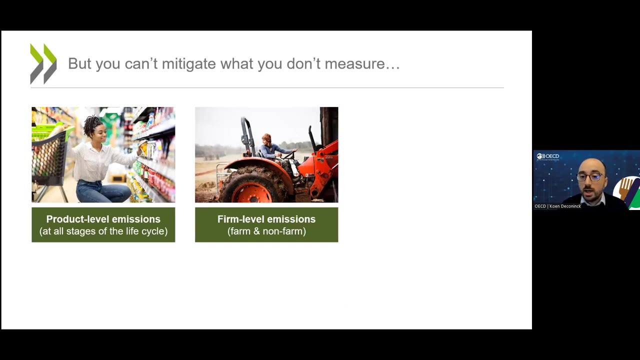 measure. any approach requires good data. we need good information on the carbon footprint at product level at all stages of the life cycle. we need data on firm level emissions of farms and other companies along the supply chain, and we need good information on the impact of our actions. in other words, what we need are: 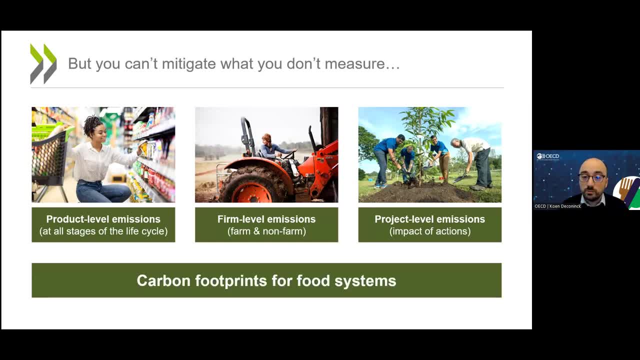 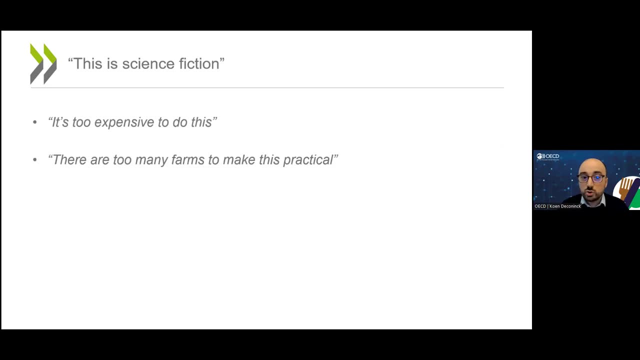 consistent, reliable, transparent carbon footprints for food systems. and maybe you're listening to this and you're thinking: good luck with that. this is science fiction, because surely it's too expensive to do this. there are so many farmers. how can we make this work? it's unclear what we 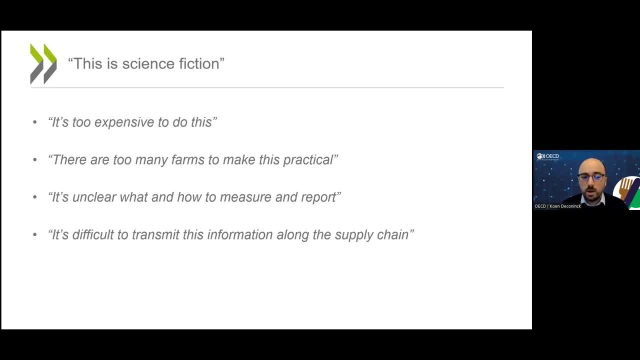 should measure, how we should measure it, how we should report it. it's difficult to transmit information along the supply chain, and is anybody really waiting for all that information? we'd like to question those assumptions. over the past few months, as we have been looking more and more, 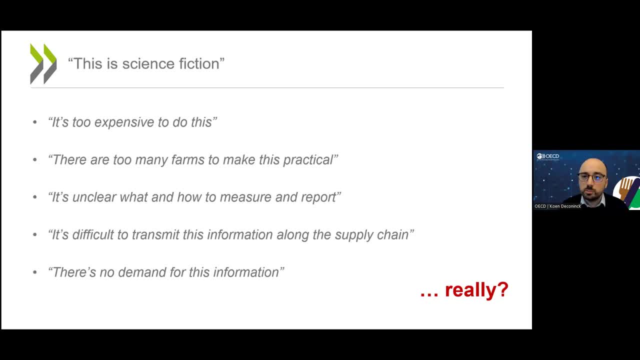 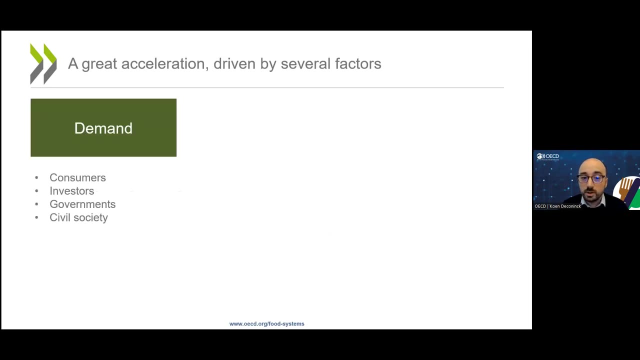 closely at this question of measuring and communicating carbon footprints in food systems. we're beginning to suspect that what we are seeing is a great acceleration, driven by several factors. first, the demand for carbon footprint information in food systems is increasing. second, it's becoming easier to supply this information, and there are also some other contextual factors that are making 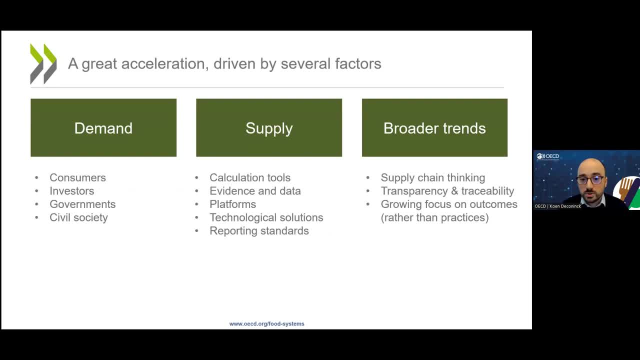 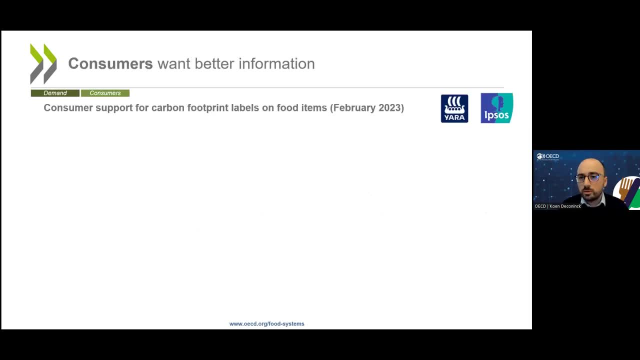 it easier to do carbon footprint reporting in food systems. i'll highlight just a few of these drivers. now, on the demand side, consumers want to make sure that their food systems are as good as they should be. a recent survey asked consumers in european countries whether they want carbon footprint. 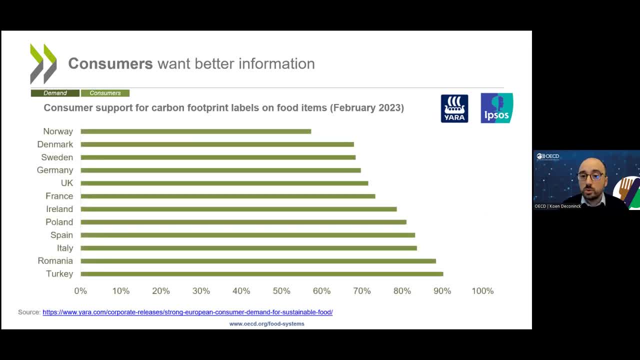 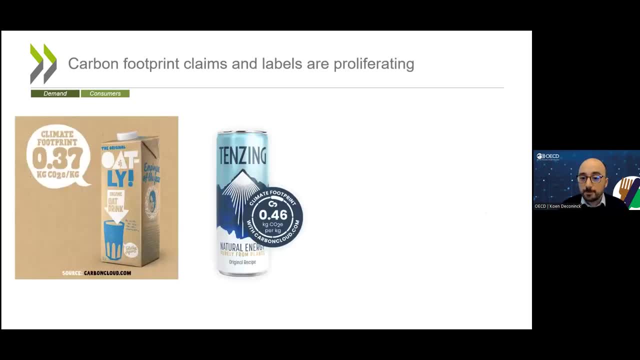 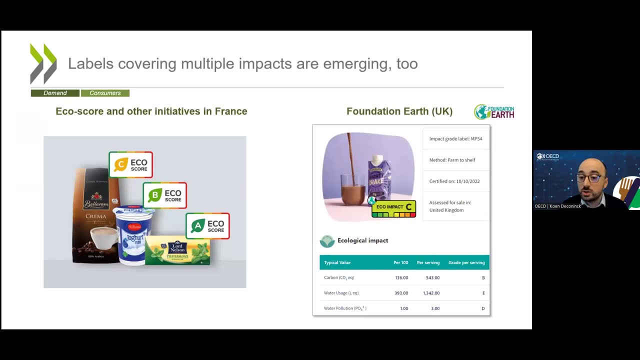 labels on food items. an overwhelming majority said yes, and indeed in the supermarkets we do see carbon footprint claims and labels emerging, and we also see other initiatives that try to communicate the environmental impacts across a range of dimensions, such as the eco score in france and the foundation earth scheme in the uk. 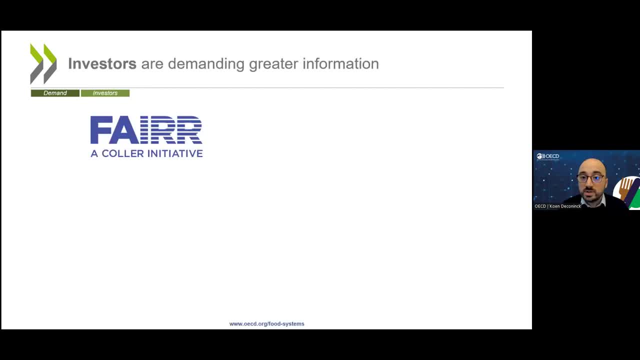 but it's not just consumers. investors are increasingly demanding greater information as well. for example, the fair initiative brings together major investors, which together represent 70 trillion dollars of assets under management. they are putting pressure on animal protein companies to provide greater transparency on their environmental impacts, and not just for 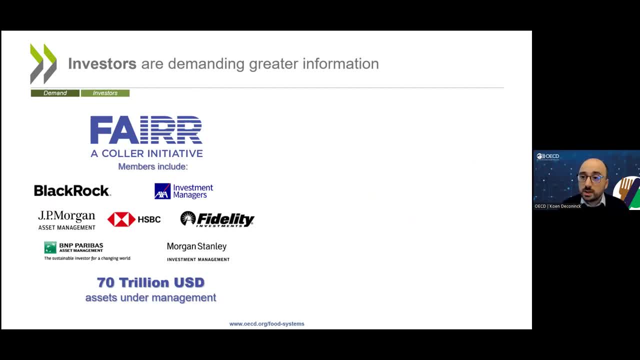 altruistic reasons. the investors consider that if governments introduce stricter rules, these could impose financial costs on those companies and at the moment they don't feel that they have enough information to judge those risks. so they are demanding greater transparency, in part because they want to minimize their own risks and maximize their profits. 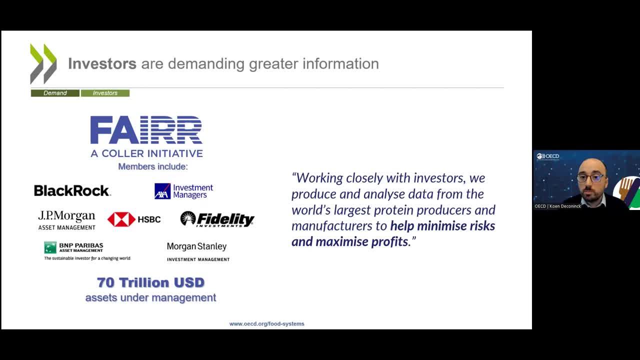 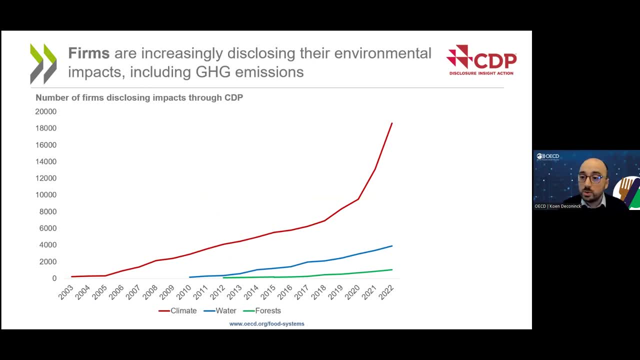 and in part due to pressure from investors. companies are indeed increasingly disclosing their environmental impacts, including greenhouse gas emissions, for example through the cdp platform. as you can see here, the number of companies across all sectors who disclose their greenhouse gas emissions through cdp has been growing exponentially over the last few years. 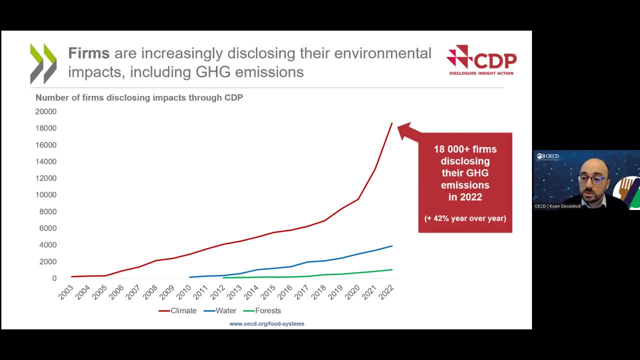 last year, more than 18 000 firms disclosed their greenhouse gas emissions. this was a 42% increase over the previous year, and these are not small companies either. they represent something like two-thirds of global stock markets. at the same time, agri-food companies are lagging somewhat behind. 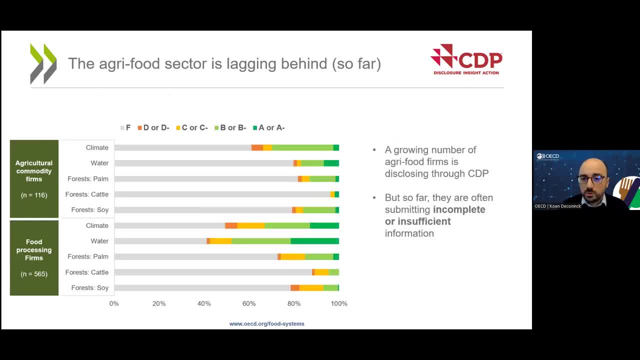 that is to say, many companies are reporting, but often the information they are providing is incomplete or insufficient according to the quality grading system used by CDP. But there is progress, For example, because firms are increasingly asked to report their scope 3 emissions. 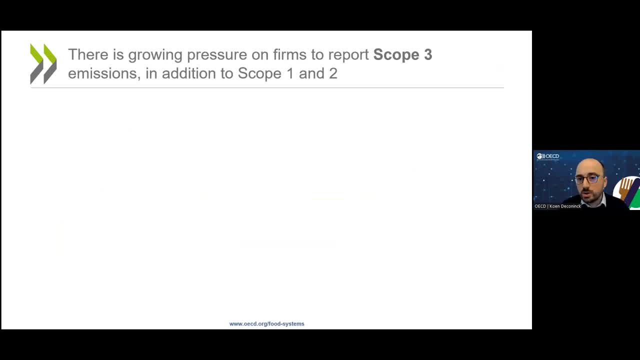 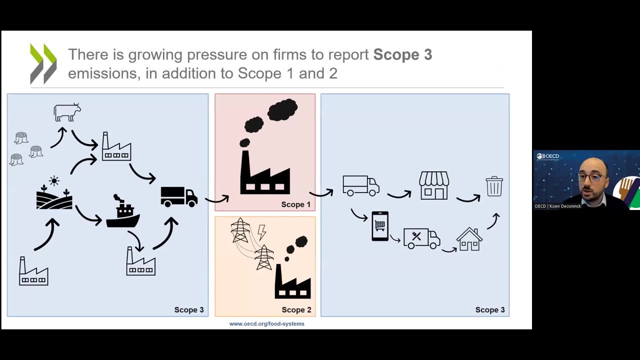 What are scope 3 emissions? Well, scope 1 emissions refer to the emissions of a company's own activities. Scope 2 are the emissions related to the energy the company is buying. Scope 3 means the emissions from the supply chain, both upstream and downstream from the firm. 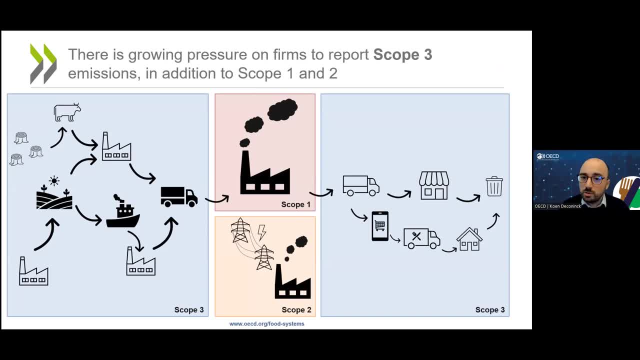 So if you are a supermarket, then the agricultural emissions of the food you are selling are part of your scope 3 emissions And retailers are indeed increasingly reporting their scope 3 emissions, and not just reporting but also setting targets to reduce those scope 3 emissions. 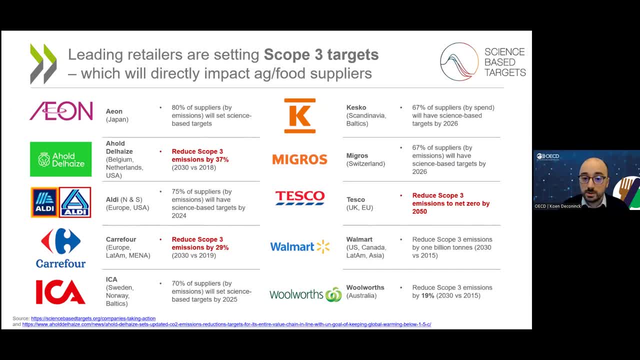 As you can see here, for some of the world's largest retailers. Given this push to reduce scope 3 targets, this will in turn put pressure on agri-food suppliers And because of that, there will also be a greater demand for information on carbon footprints. 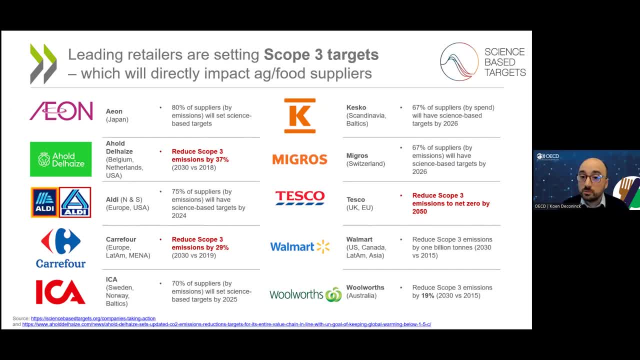 So this is one source of the demand for greater information on carbon footprints. Another source of the demand is, of course, public policy, And in the end the demand for information on carbon footprints is increased by 20%. So this is one source of the demand for greater information on carbon footprints. 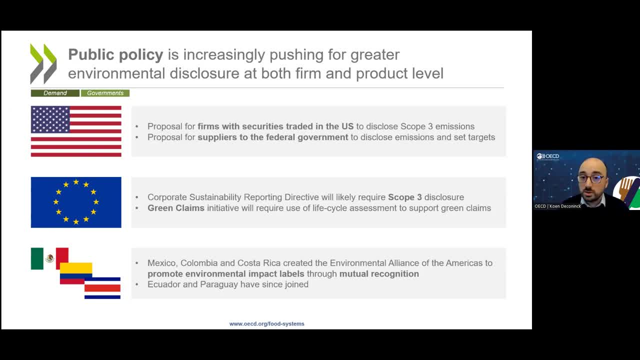 In many jurisdictions, governments are pushing for greater environmental disclosure. For example, both in the United States and in the European Union, there are proposals that would essentially require most large firms to report their Scope 3 emissions, And both in Europe and in Latin America we see initiatives to promote labels that communicate environmental impacts. 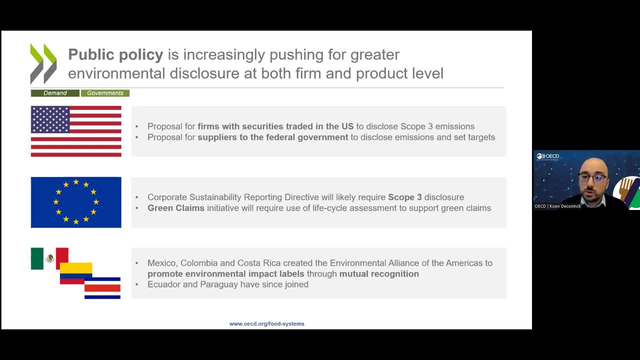 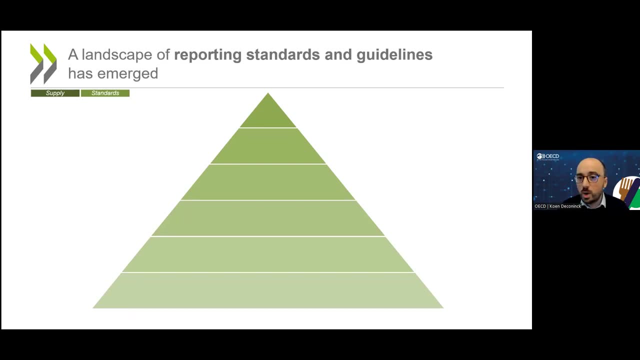 At the same time, as I mentioned earlier, it's also becoming easier to supply carbon footprint information. A large part of the story there is that over the last few years, a landscape of reporting standards has emerged. If you're new to this, it can seem quite intimidating, but it's best to think of it as a pyramid, ranging from the more general to the more specific. 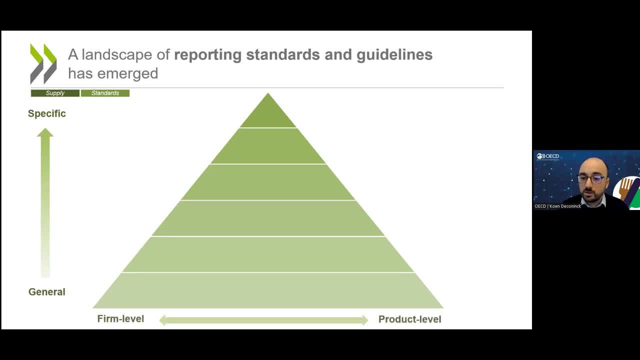 And we can also differentiate between more firm-level and more product-level standards. For example, there are standards on sustainability reporting, such as those of the Global Reporting Initiative, and standards which are currently being developed by IFRS, which is the body that also sets global financial accounting rules. 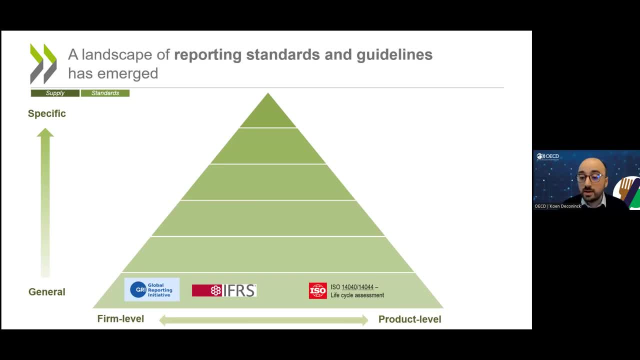 At the product level, ISO has a widely used standard for lifecycle assessment which covers multiple environmental impacts. The next step of the pyramid is specifically about greenhouse gas emissions. The two major organizations here are the Greenhouse Gas Protocol and ISO, and both have standards for firm-level reporting and for product-level carbon footprint. 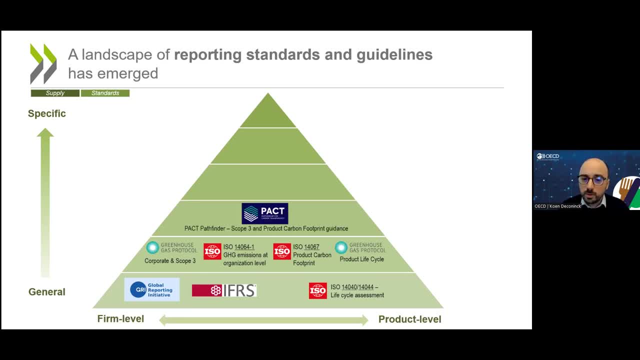 I also want to highlight the work of the PACT Pathfinder Initiative. PACT Pathfinder tries to provide much clearer guidance on product-level carbon footprints to in turn, make it easier for companies to report their Scope 3 emissions. So you could see this as building a bridge between the product-level and firm-level reporting. 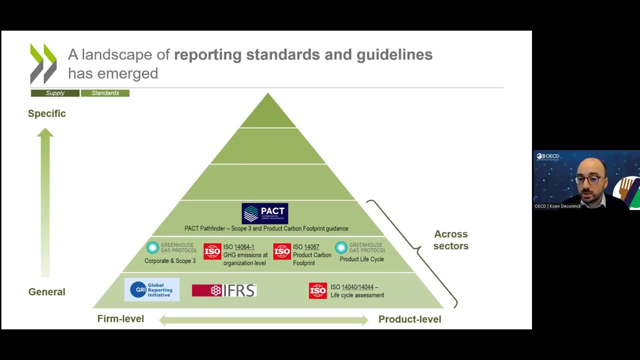 All of these are sector-agnostic, not sector-specific, but we can also distinguish the ones that are specific for agriculture and food and build on top of this. For example, the Greenhouse Gas Protocol has guidance for the agricultural sector and is currently developing more guidance for the land sector. 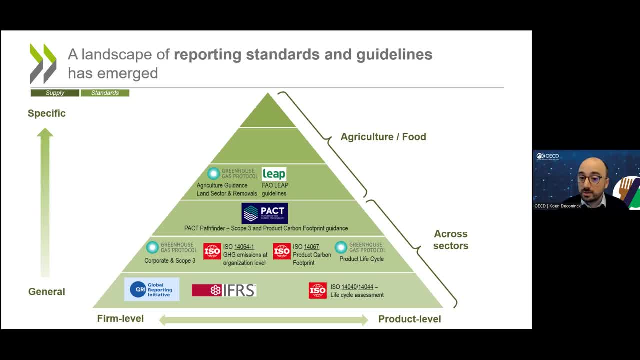 FAO is also managing the LEAP project, which is providing guidelines on the environmental assessment of livestock. We can get even more specific. For example, there exists specific guidance for the US dairy sector, which builds on the Greenhouse Gas Protocol. 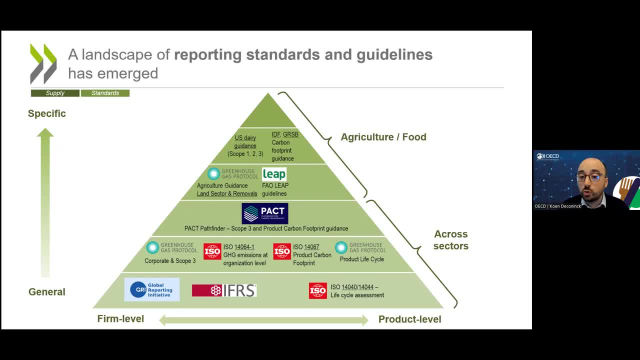 And both the International Dairy Federation and the Global Roundtable for Sustainable Beef have produced guidance on this. We also have guidance on carbon footprints, And that brings us all the way to the top of the pyramid, because there is still one piece missing here. And that is the actual numbers. If there is a cow in a field somewhere, how much methane did it actually emit? Ideally, we would have direct measurement to answer that question, But in practice that is not what is commonly done, because it's very difficult to measure these things directly. 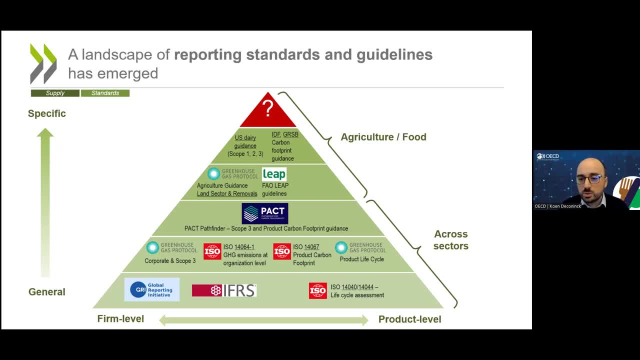 So instead, people use calculation tools, And how this works is that calculation tools are often built on detailed scientific models that are then simplified so that farmers can simply provide some key performance indicators from their farm and obtain a reasonably accurate estimate of greenhouse gas emissions. 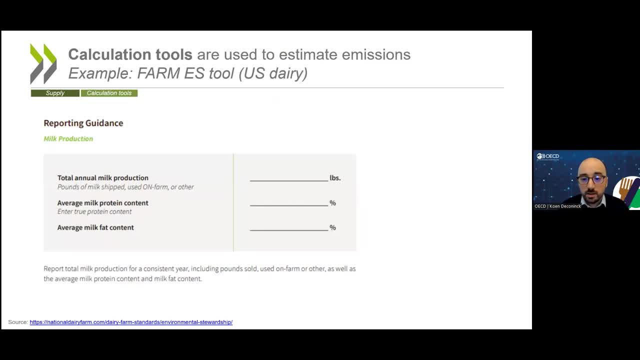 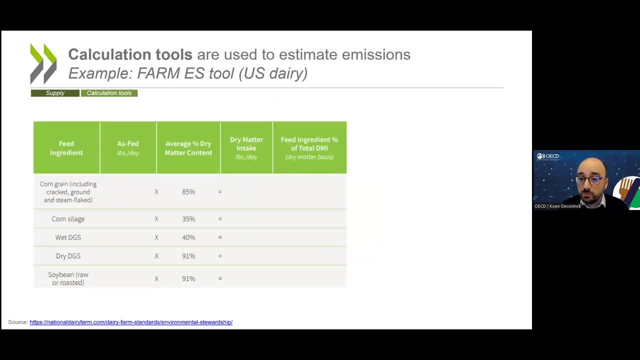 Here's an example from the United States. Farmers can provide information on how much milk they produce, on how many cows they have, on what kind of animal feed they are using and what kind of manure management approach they have in place, and some other bits of information. 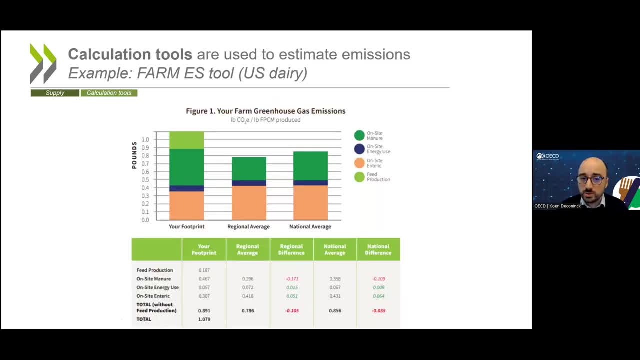 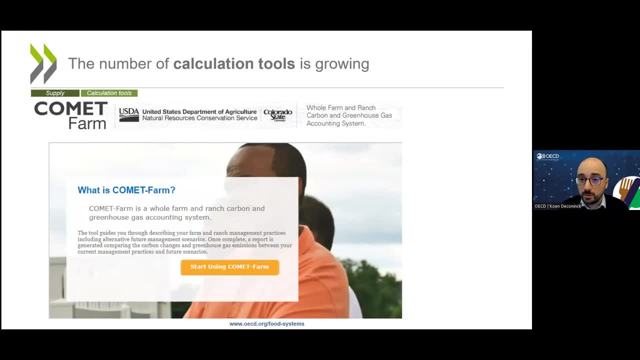 And then the tool provides an estimate of greenhouse gas emissions. This is just one example. There are many other calculation tools out there, such as the Cool Farm tool and the Comet Farm tool. What is attractive about calculation tools is also that they allow us to really scale up carbon footprints. 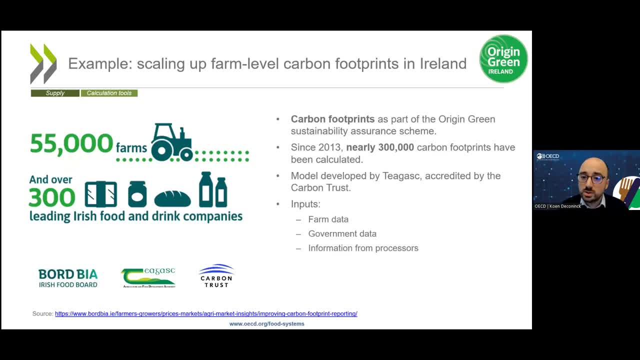 And a great example here comes from the Origin Green scheme in Ireland, which is a sustainability assurance scheme, And as part of the scheme, since 2013, they have been using a carbon footprint calculation tool to come up with nearly 300,000 carbon footprint estimates for their farmers. 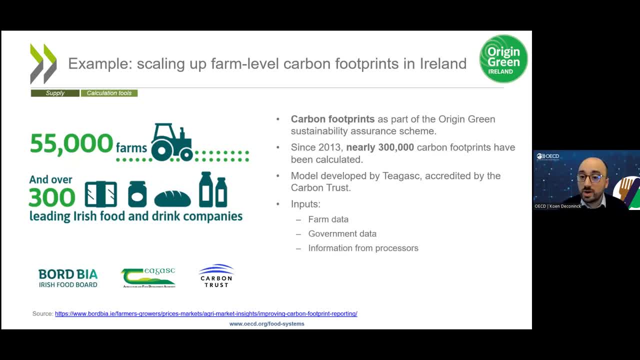 which means that many farmers now have multiple data points to track their progress over time. Ideally, we use as much primary data as we can when we're coming up with carbon footprints for food systems, but that is not always possible. Sometimes we need to fill the gaps. 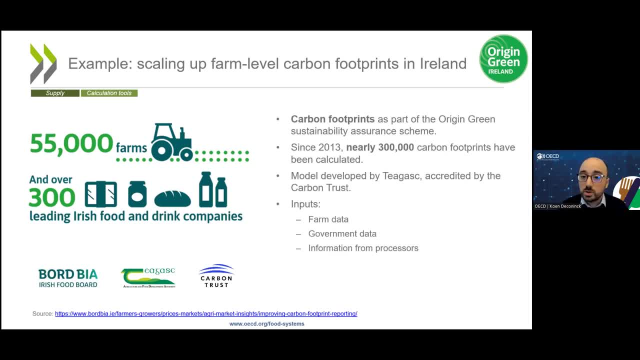 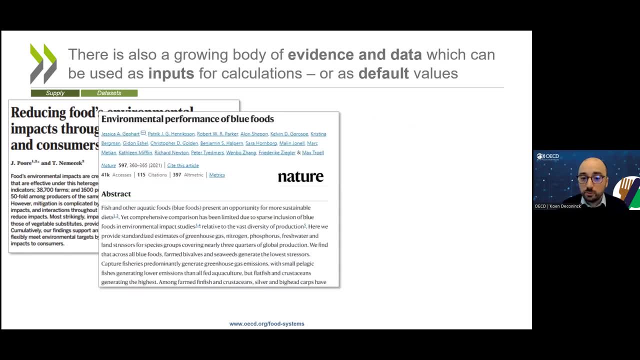 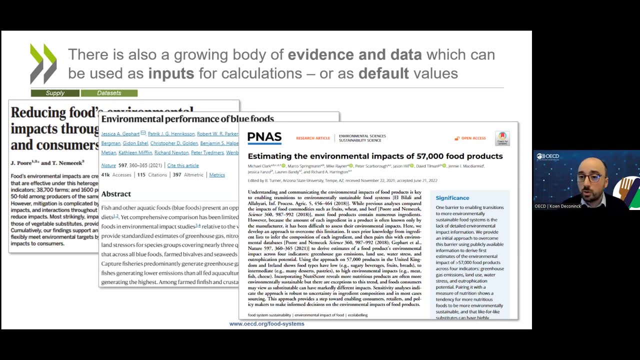 Even this is becoming easier, however, Because of the growing availability of evidence and data. For example, there have been some major impactful scientific studies recently which have really advanced our understanding of the environmental impacts of food products. There are also other databases collecting information on lifecycle assessments. 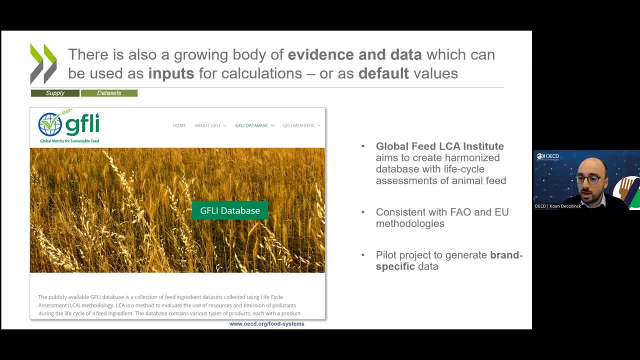 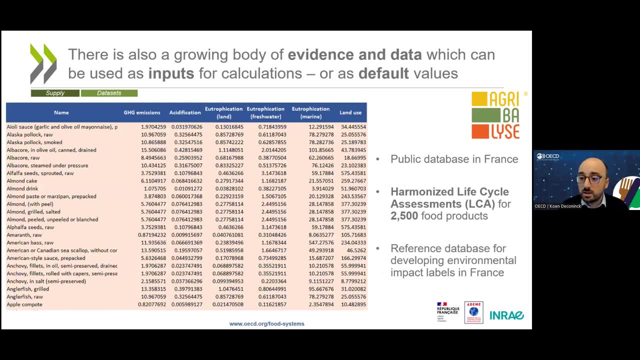 such as the Global Feed LCA Institute, which collects lifecycle information on animal feed, And, in France, the Agribalise project, a public database with lifecycle assessments for nearly 2,500 food products, And, as you can see here, that covers greenhouse gas emissions. 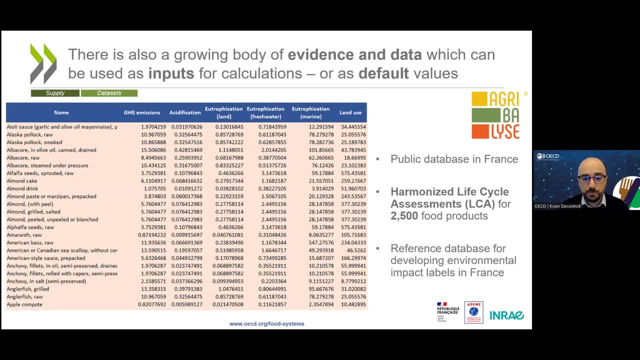 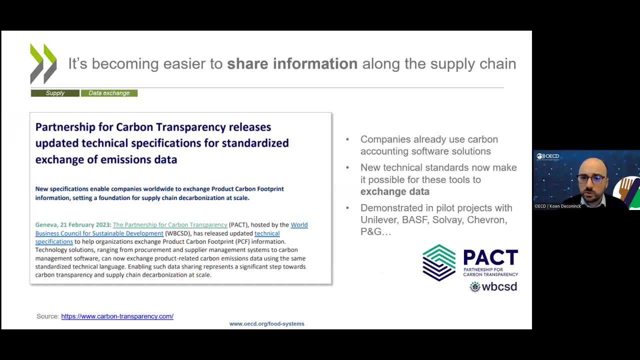 and several other environmental impacts as well. It is also becoming easier to share information along the supply chain, And there are many initiatives underway here, but I just want to highlight one. Large companies often already use some form of carbon accounting software for internal calculations and for some external reporting. 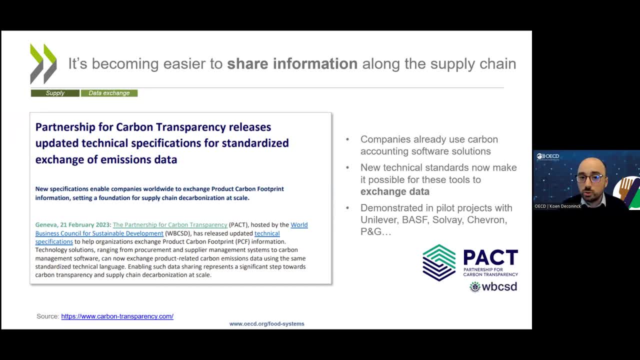 But until recently, software packages from different vendors could not communicate with each other. The Partnership for Carbon Transparency brought industry players together to agree on a common technical standard to make it possible to communicate between these different software packages, And they demonstrated this in pilot projects with major multinationals. 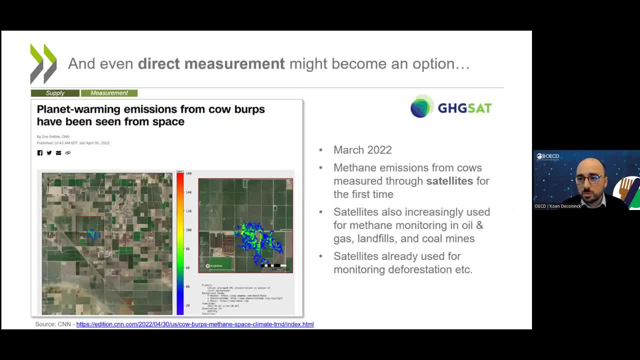 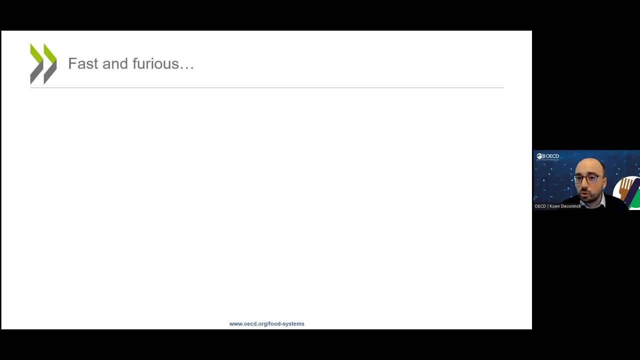 I mentioned earlier that direct measurement is difficult, but even that might now be changing. Last year, a company announced that they had used satellites to measure methane emissions from cows, So we are truly entering a brave new world of measuring and communicating environmental impacts and especially carbon footprints in food systems. 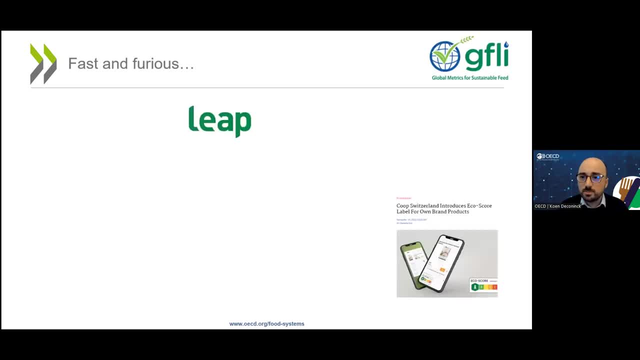 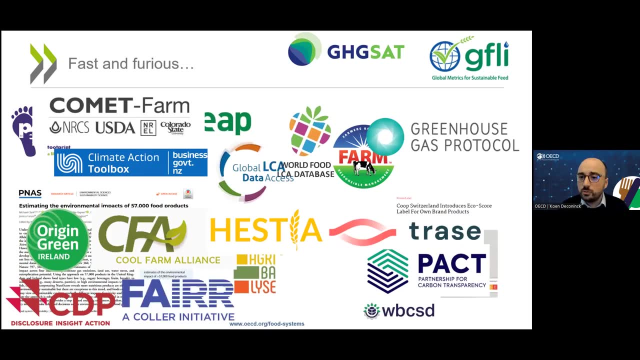 Or, as we like to call it, fast and furious. Fast because there is rapid progress in this space, but also furious because we see a confusing landscape of initiatives screaming for our attention. And, on the one hand, it's great to see all this activity. 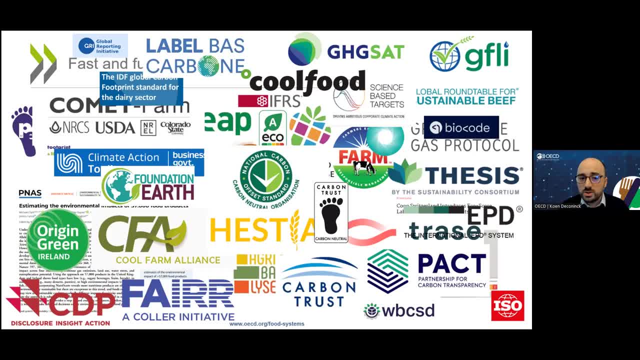 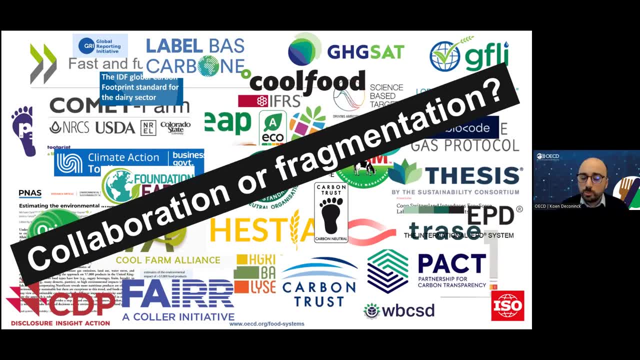 But on the other hand, it does raise the question: are we seeing collaboration or fragmentation? Imagine a situation where there are many different reporting standards, many different calculation methodologies, a situation where every country or even every supermarket has a different labeling scheme and different requirements on suppliers. 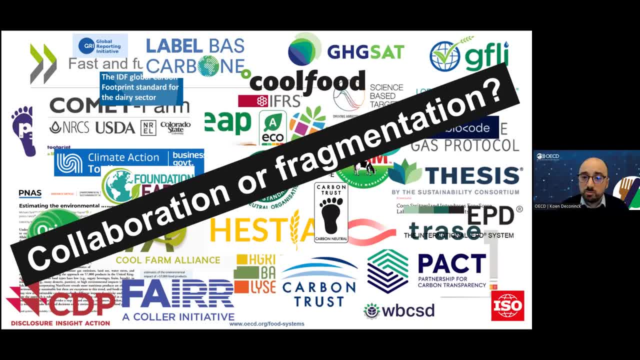 In that situation we would have massive administrative burdens and barriers to trade. First of all, it doesn't seem likely that we would actually achieve lower emissions with all that fragmentation, So it would really be the worst of both worlds. But it doesn't have to be that way.